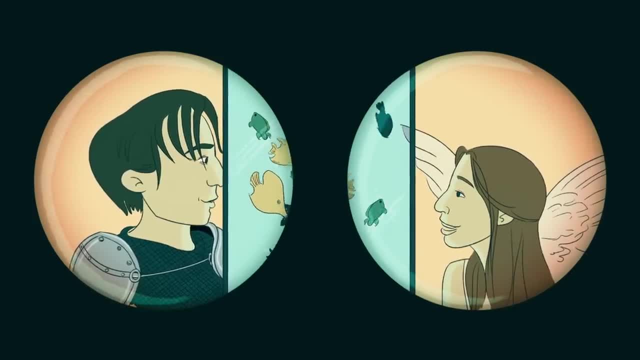 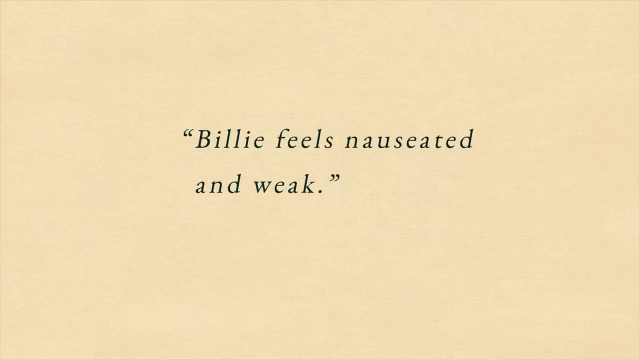 We see and hear the interactions of the characters and the setting, But with prose fiction, all you have is static symbols on a contrasting background. If you describe the story in matter-of-fact, non-tactile language, the spell risks being a weak one. 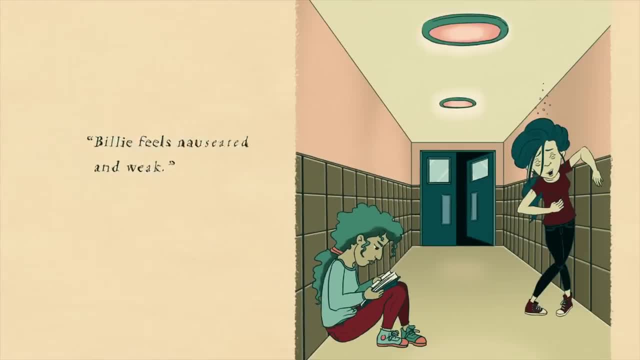 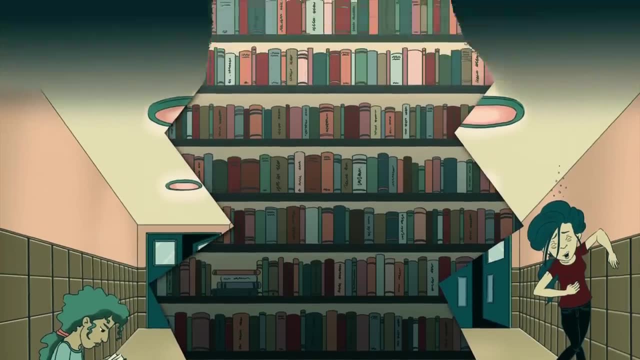 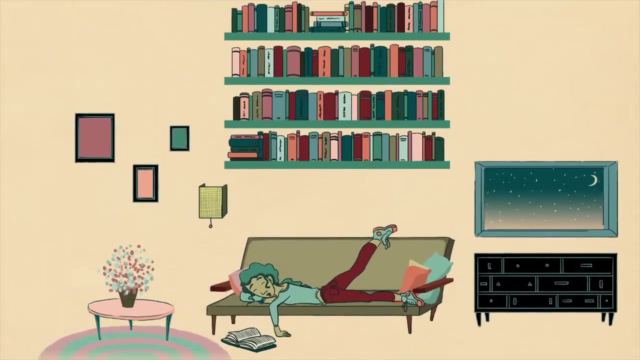 Your reader may not get much beyond interpreting the squiggles. She will understand what Billy feels like, but she won't feel what Billy feels. She'll be reading, not immersed in the world of the story, discovering the truths of Billy's life at the same time that Billy herself does. 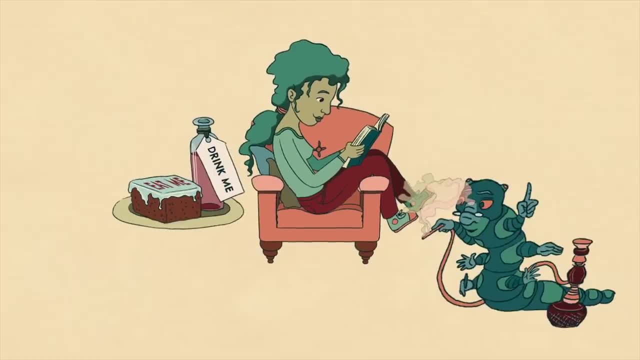 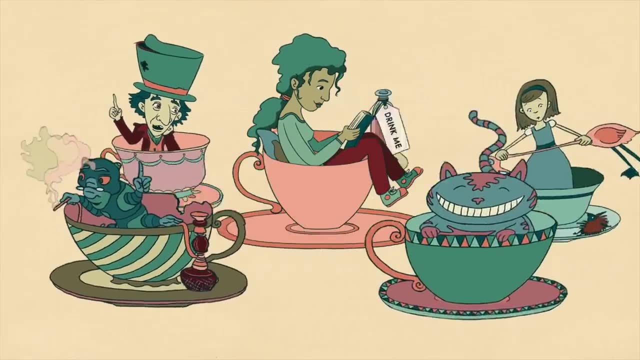 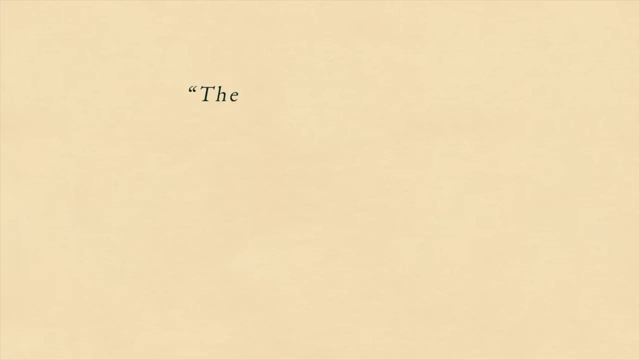 Fiction plays with our senses: Taste, smell, touch, hearing, sight and the sense of motion. It also plays with our ability to abstract and make complex associations. Look at the following sentence: The world was ghost-quiet, except for the crack of sails and the burbling of water against hull. 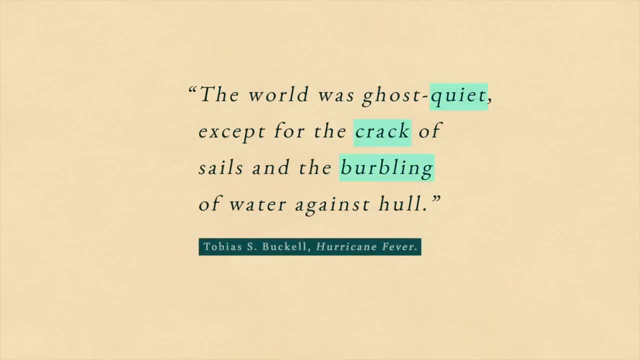 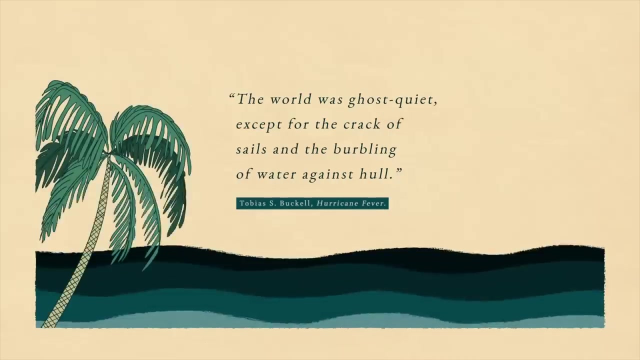 The words quiet, crack and burbling engage the sense of hearing. Notice that Bacall doesn't use the generic word sound. Each word he chooses evokes a particular quality of sound. Then, like an artist laying on washes of color to give the sense of tension. 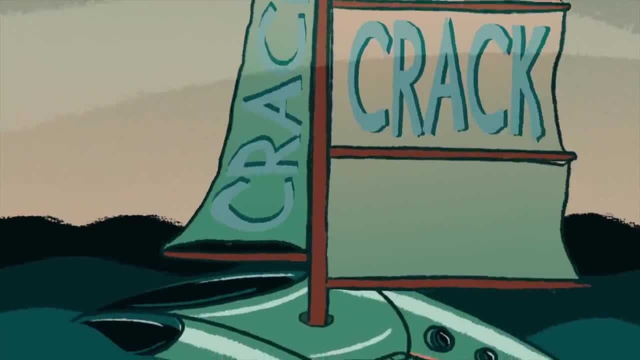 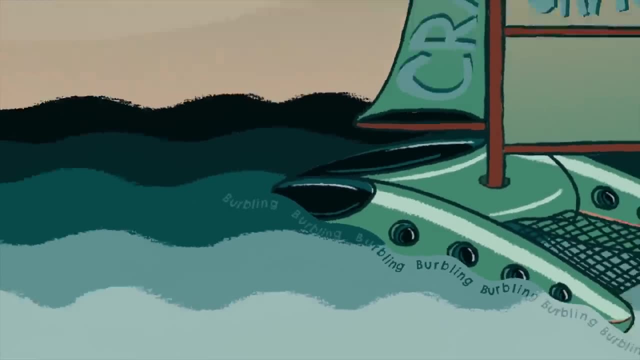 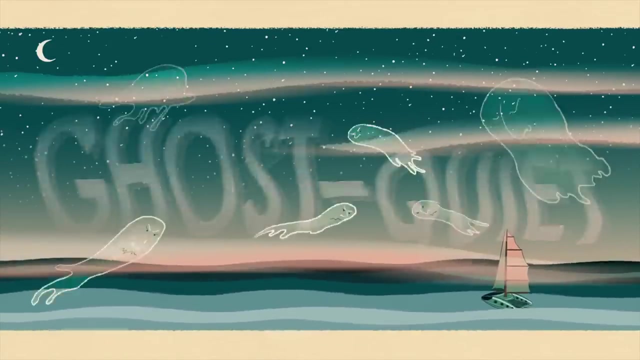 he adds another layer: motion, the crack of sails and touch the burbling of water against hull. Finally, he gives us an abstract connection by linking the word quiet with the word ghost- Not quiet as a ghost, which would put a distancing layer of simile between the reader and the experience. 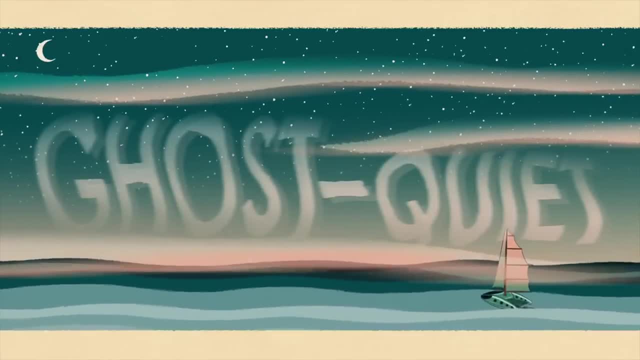 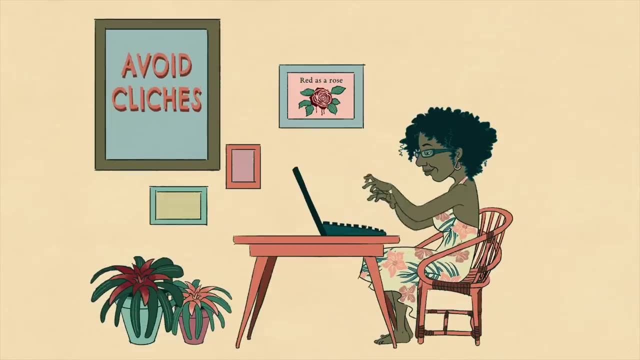 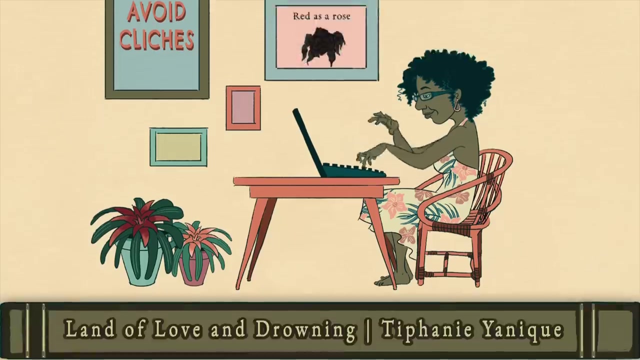 Instead, Bacall creates the metaphor ghost-quiet For an implied rather than overt Comparison. writers are always told to avoid cliches because there's very little engagement for the reader in an overused image such as red as a rose. but give them love. 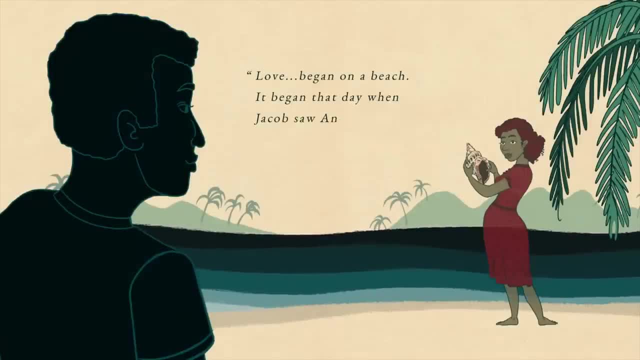 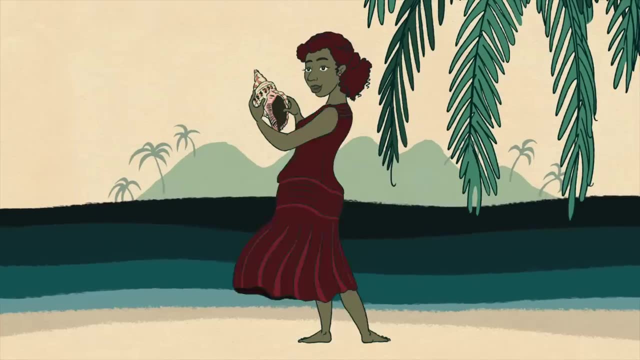 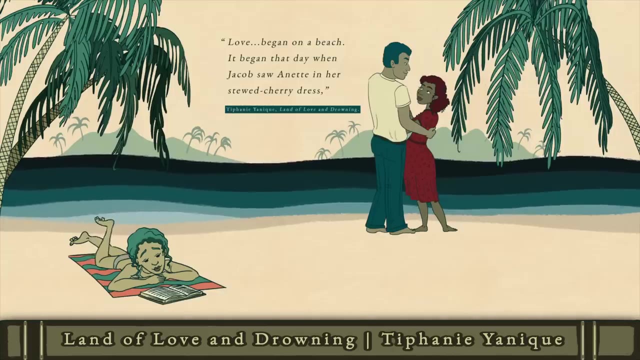 Began on a beach. it began that day when Jacob saw Annette in her stewed cherry dress, and Their brains engage in the absorbing task of figuring out what a stewed cherry dress is like. suddenly, They're on a beach, about to fall in love. They're experiencing the story at both a visceral and a conceptual level.